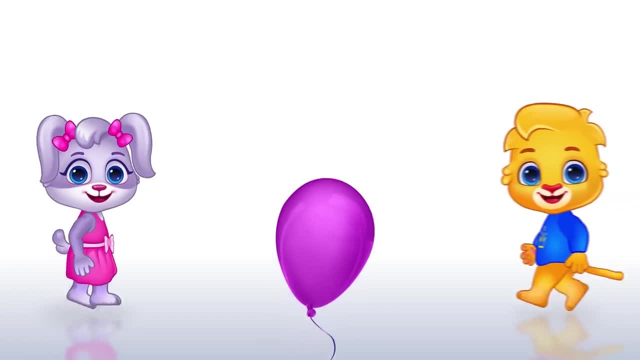 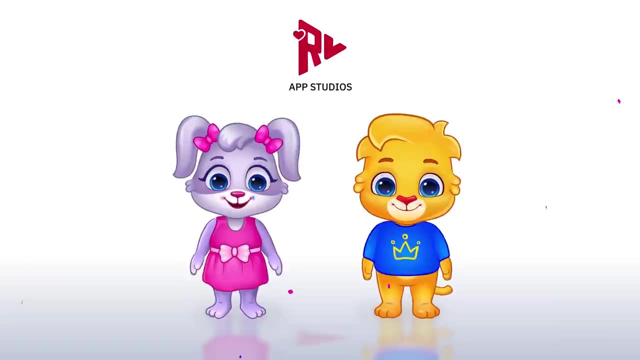 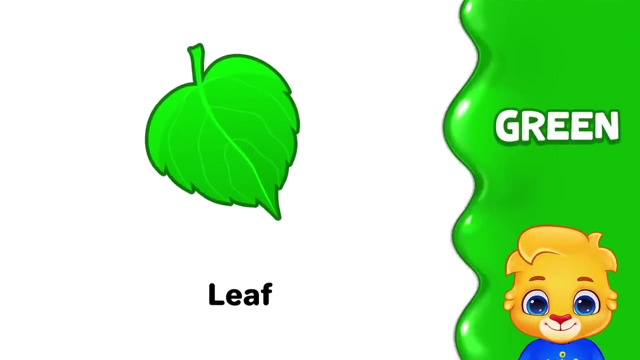 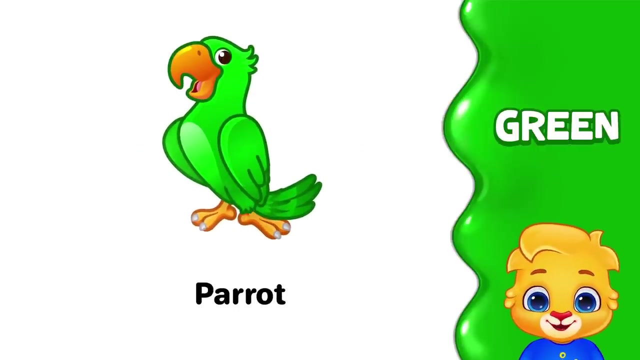 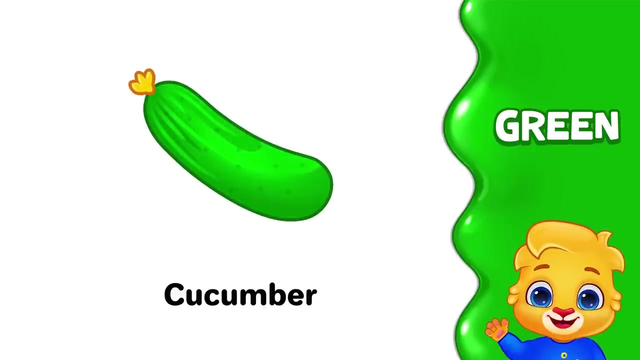 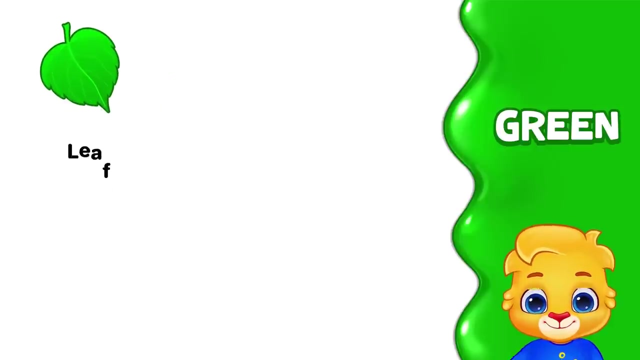 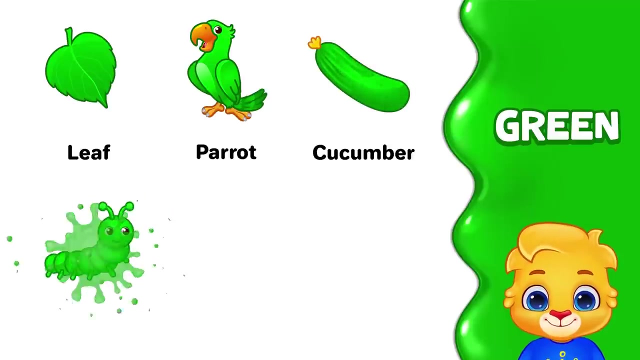 Hello. green Leaf is green, Parrot is green, Cucumber is green, Cucumber is green, Caterpillar is green, Tree is green, Watermelon is green. Green leaf, Green Parrot, Green Cucumber, Green Caterpillar. 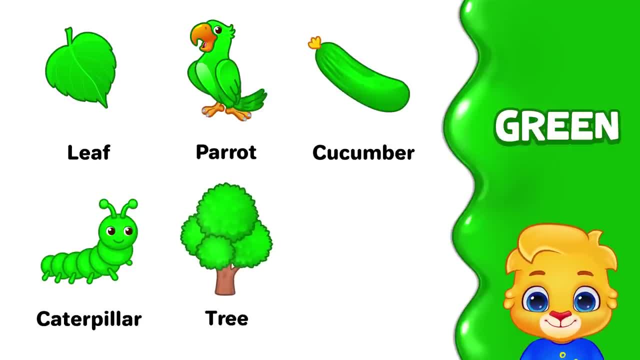 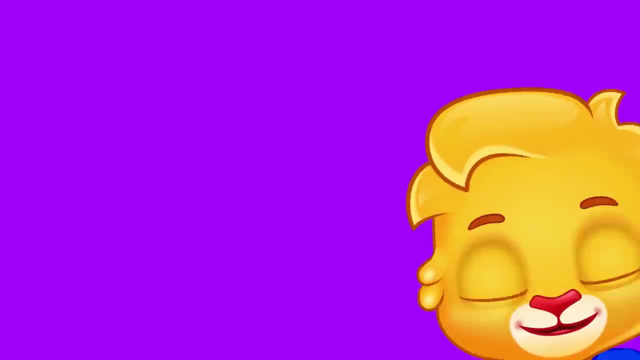 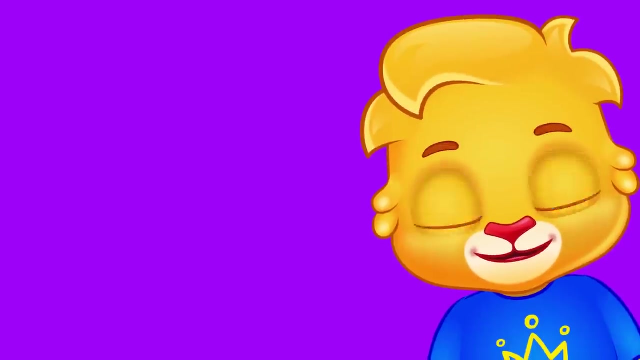 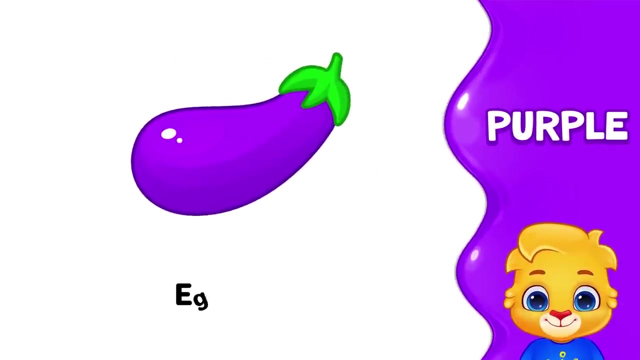 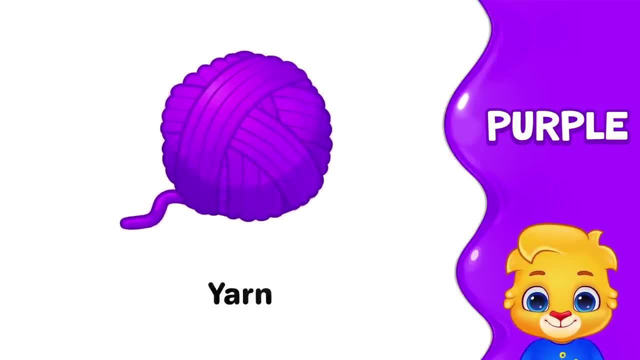 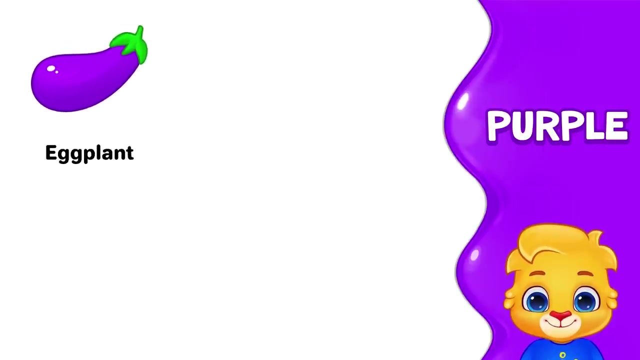 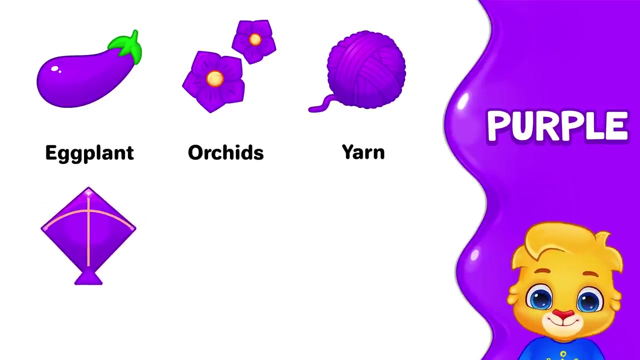 Yarn is purple. Kite is purple. Turnip is purple. Lollipop is purple. Purple is purple. Eggplant is purple. Orchids are purple. Yarn is purple. Kite is purple. Turnip is purple. Lollipop is purple. 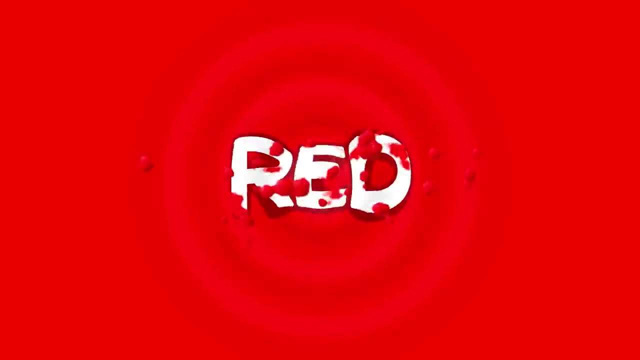 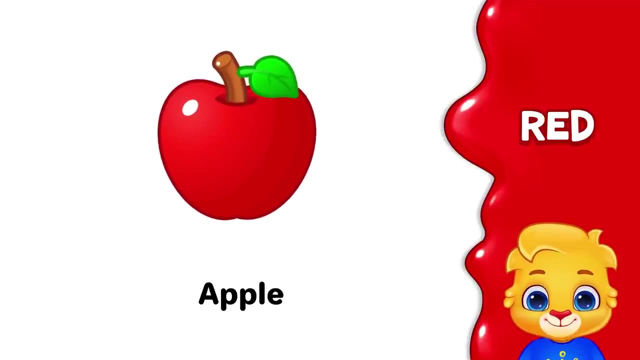 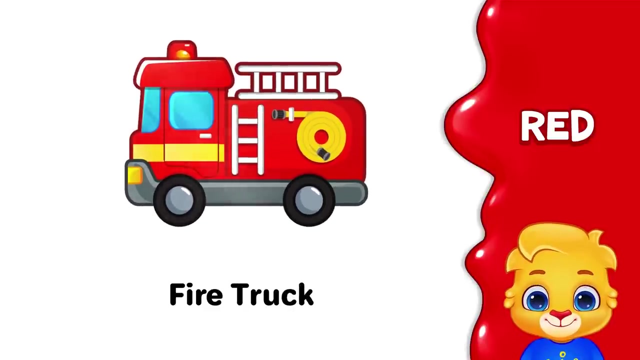 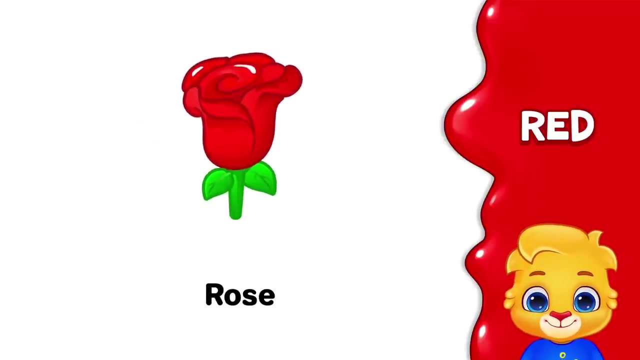 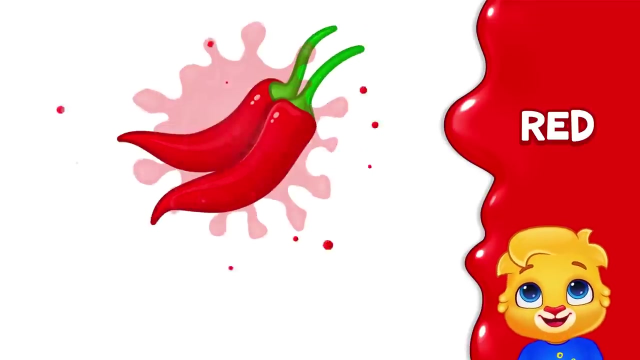 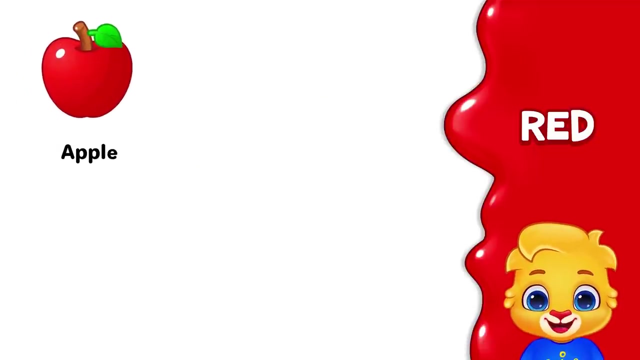 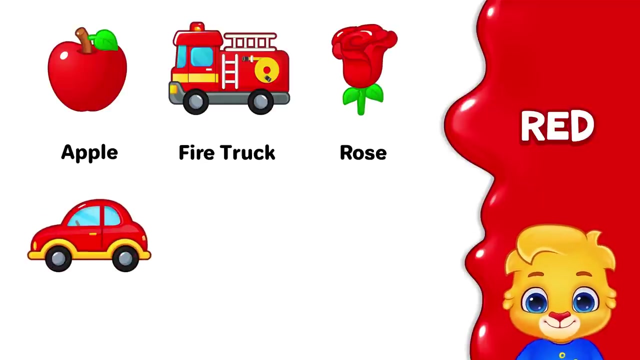 Red is purple, Red, Apple is red. Fire truck is red. Rose is red, Car is red, Strawberry is red. Strawberry is red. Red chili is red. Red. apple Red. fire truck Red rose, Red car, Red car. 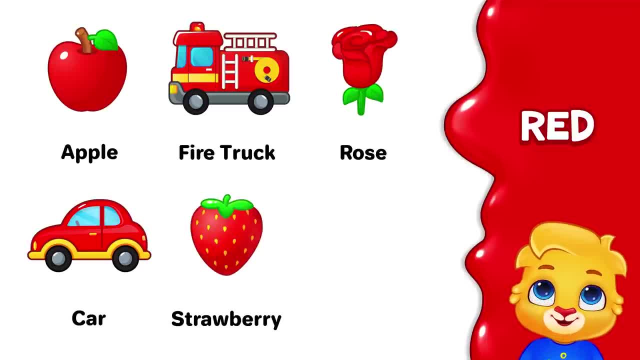 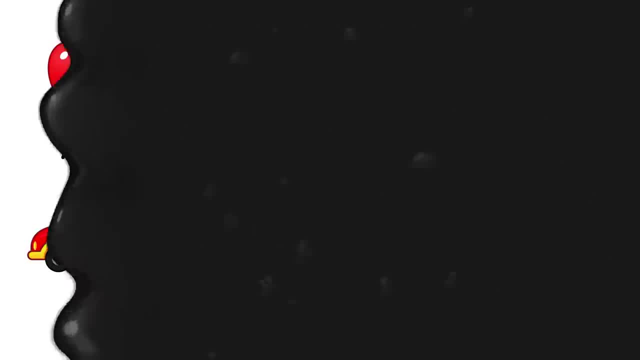 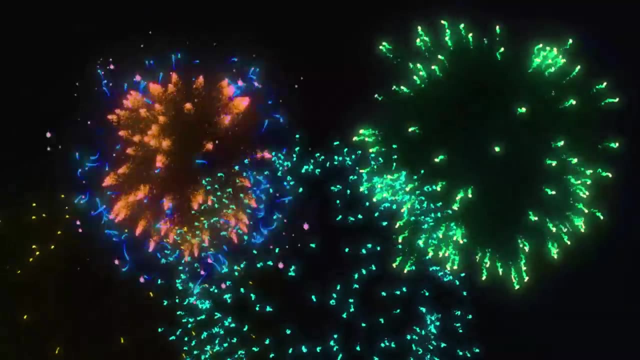 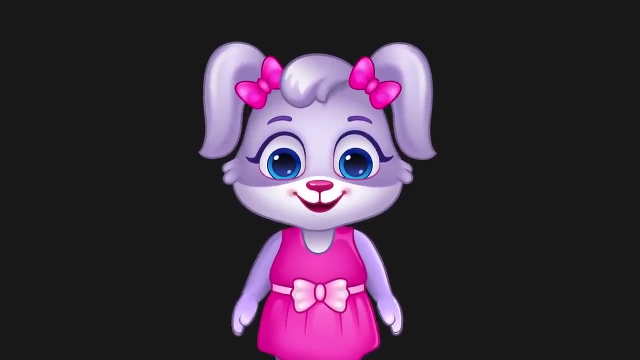 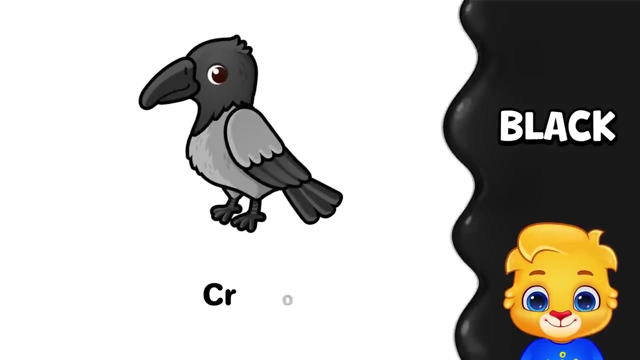 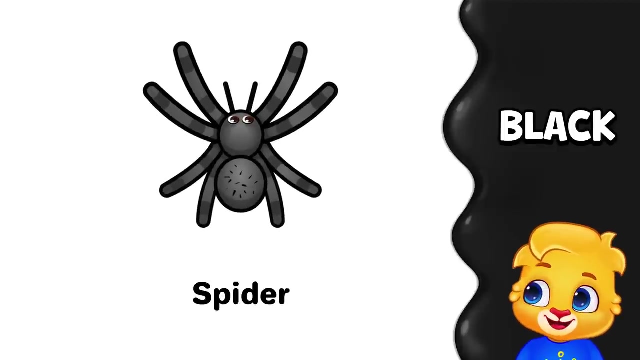 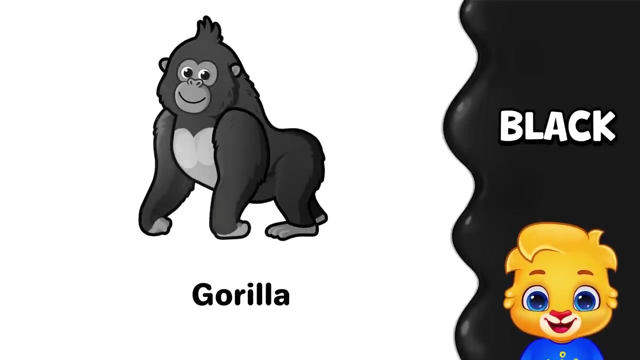 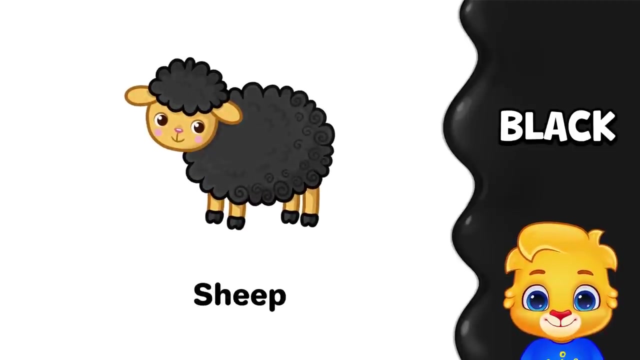 Red strawberry, Red strawberry, Red, red chili, Red red chili. Fantastic, Black Black Crow is black. Crow is black. Spider is black. Gorilla is black. Sheep is black. Sheep is black. Sheep is black. Umbrella is black. 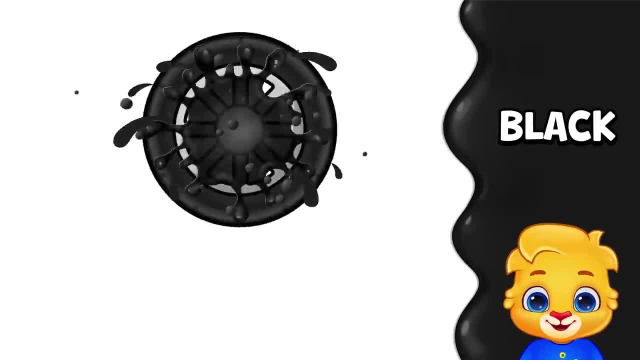 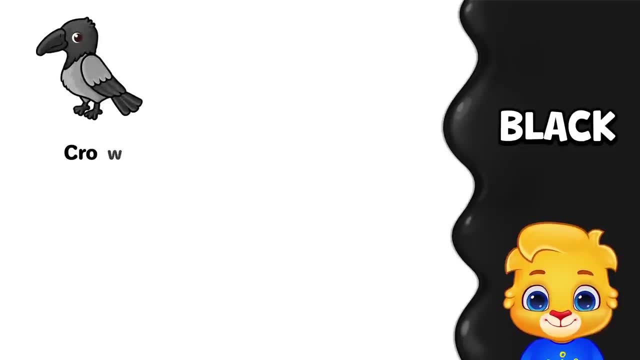 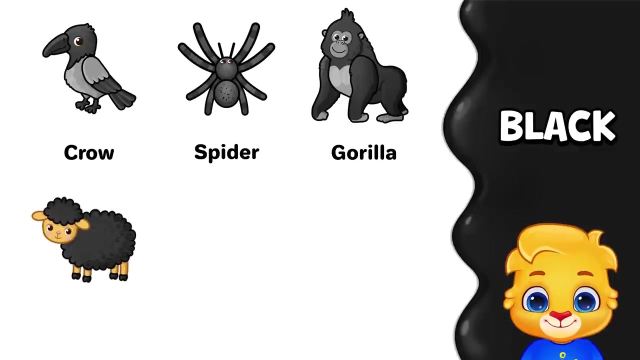 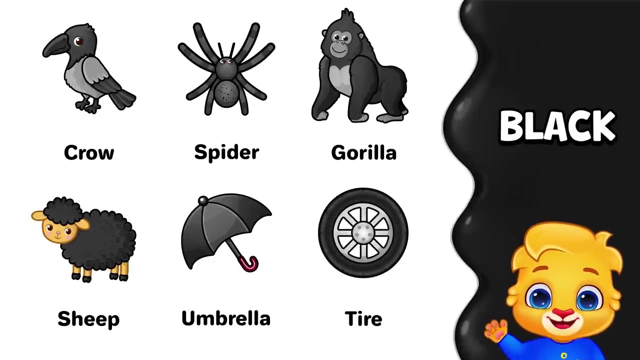 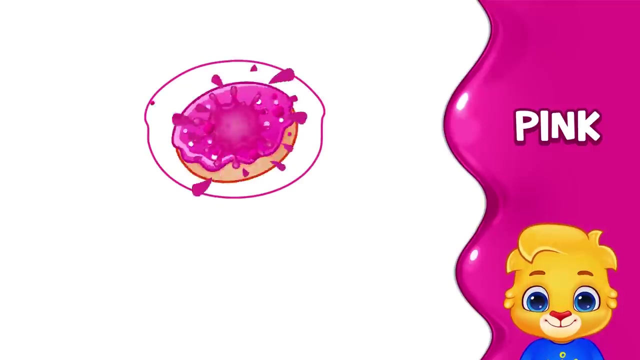 Umbrella is black, Tire is black, Tire is black, Tire is black. Crow, Crow, Spyder, Spyder, Gorilla, Gorilla Sheep, Black sheep. Black umbrella, Black tire, Pink Donut is pink. 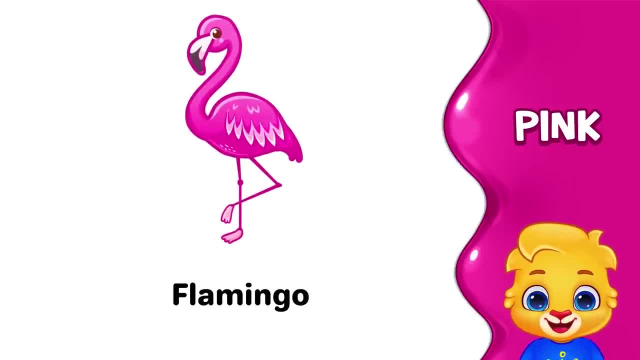 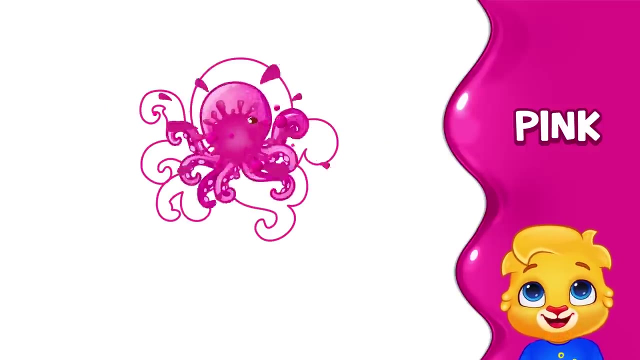 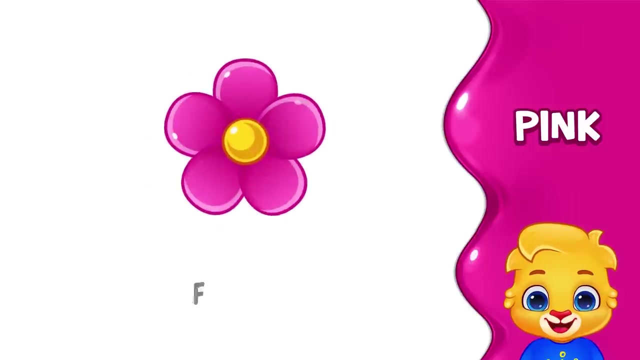 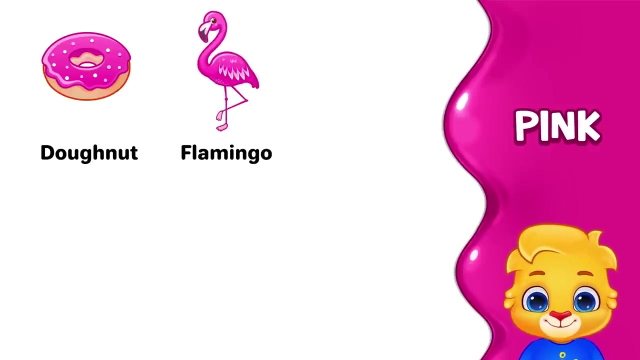 Flamingo is pink. Cupcake is pink. Pig is pink. Octopus is pink. Flower is pink. Pink Donut is pink. Pink Flamingo is pink. Cupcake is pink. Pig is pink. Octopus is pink. 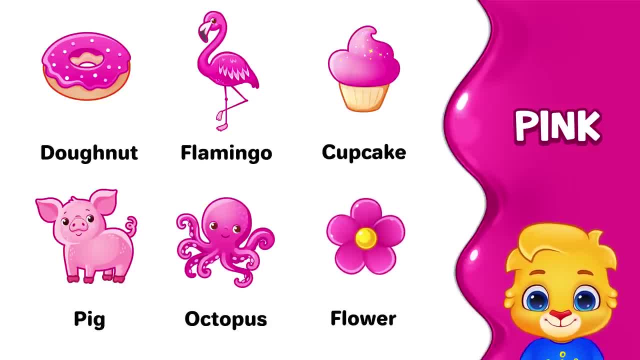 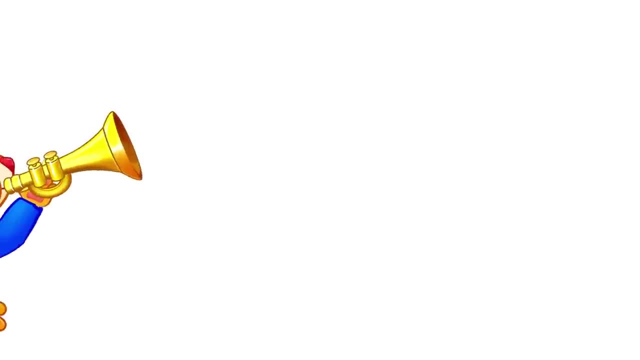 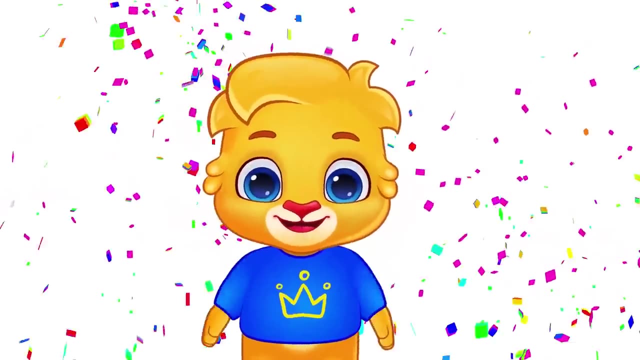 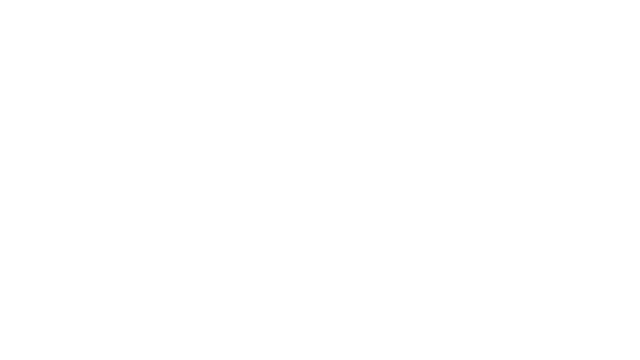 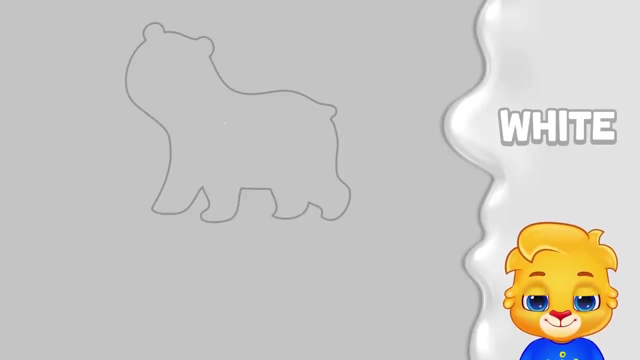 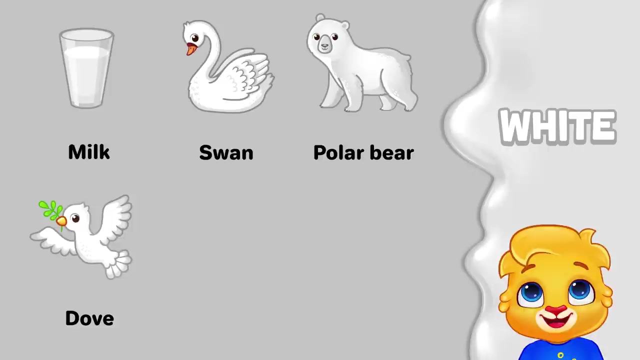 Flower is pink. Hello, my friend, Celebration for you, Bye-bye. White Juice is white. Milk is white. Swan is white. Polar bear is white. Dove is white. Snowman is white. Snowman is white is white. Egg is white. White milk, White swan White. polar bear, White dove, White. 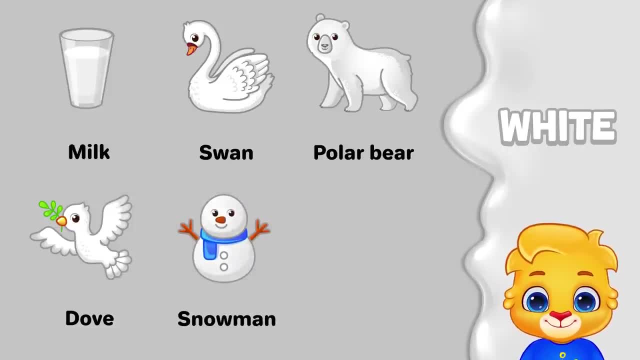 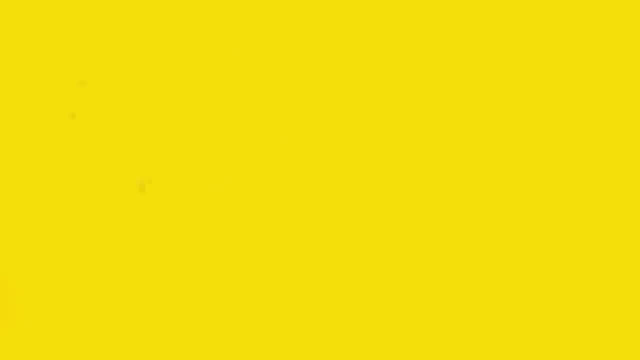 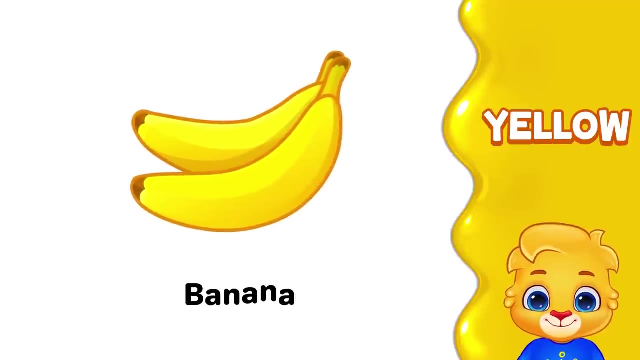 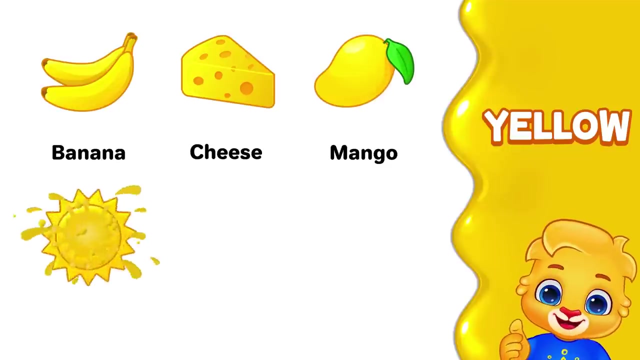 snowman White egg. Yellow Banana is yellow. Cheese is yellow. Mango is yellow. Sun is yellow. Duck is yellow. Sunflower is yellow. Yellow Banana, Yellow Cheese, Yellow Mango, Yellow Sun, Yellow Duck, Yellow Sunflower. 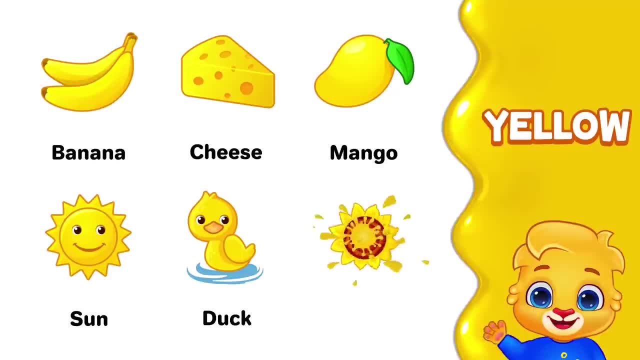 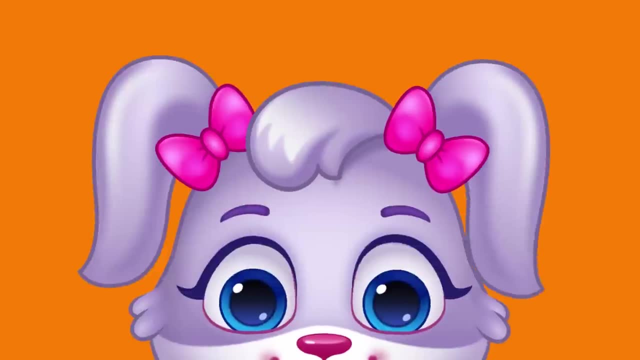 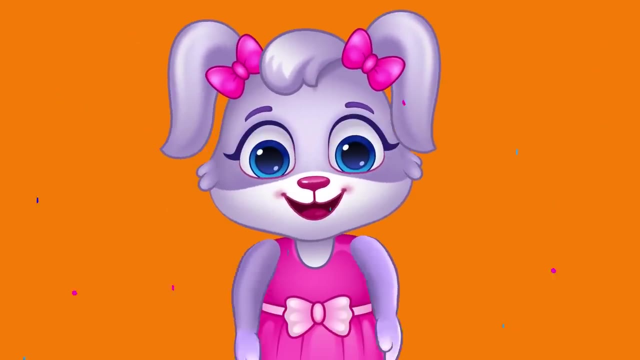 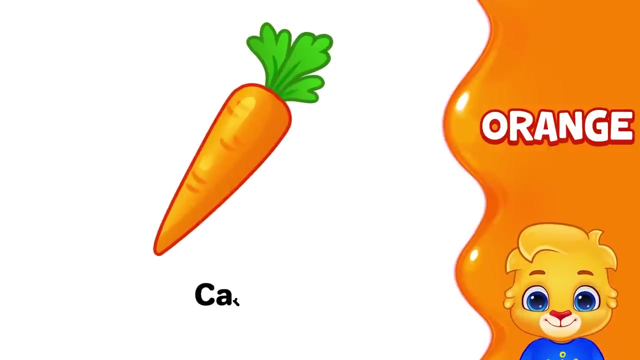 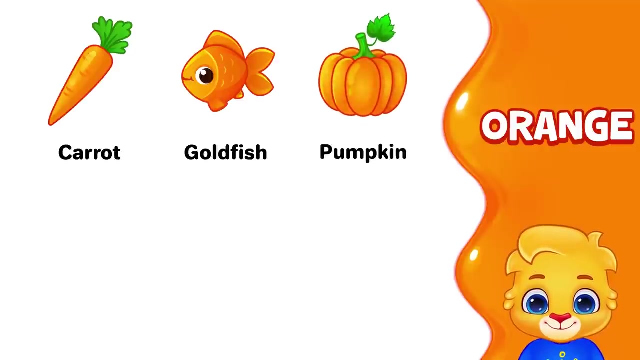 Yellow Duck, Yellow Sunflower. Orange. Carrot is orange, Goldfish is orange. Pumpkin is orange. Jelly is orange. Basketball is orange. Popsicle is orange. Orange carrot, Orange, goldfish, Orange pumpkin. Orange is orange. Orange Jelly, Orange, Basketball, Orange Popsicle. 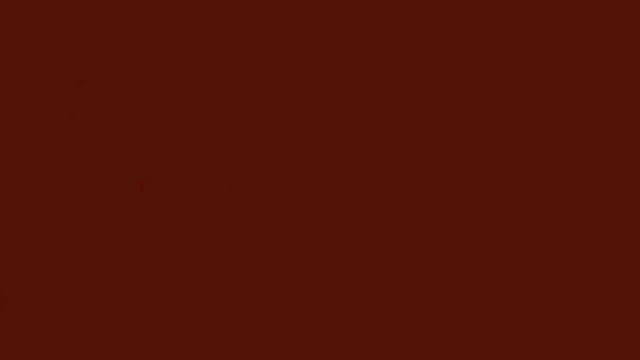 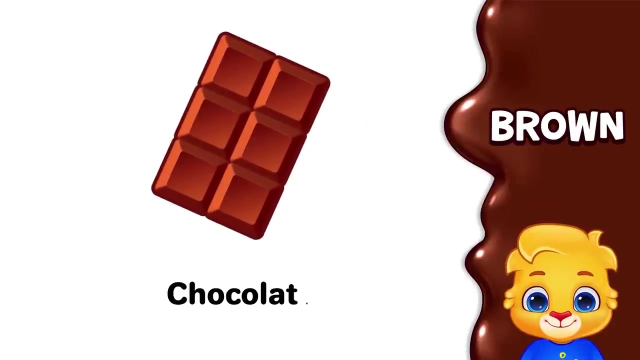 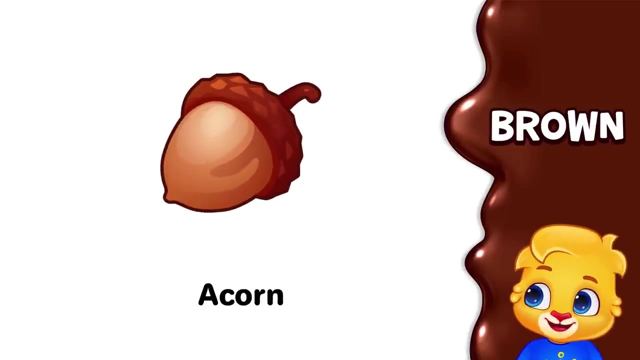 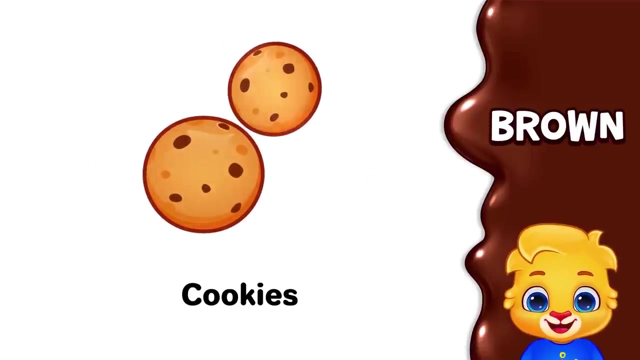 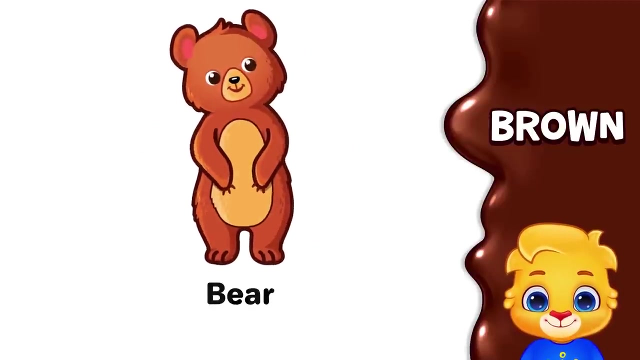 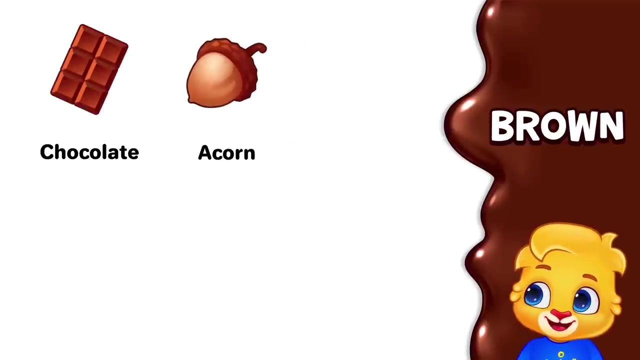 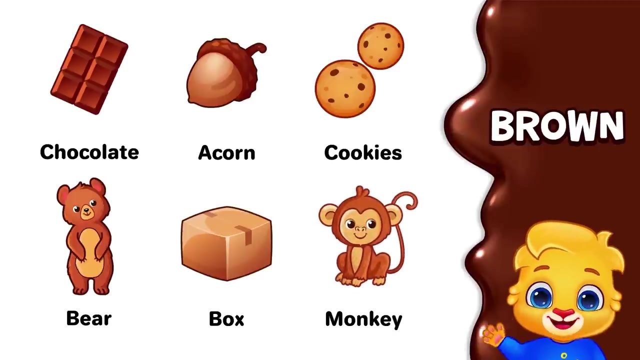 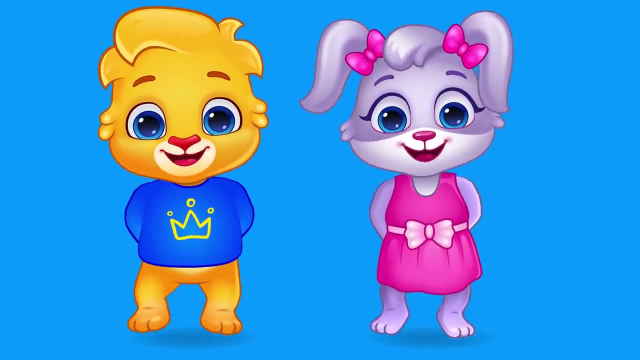 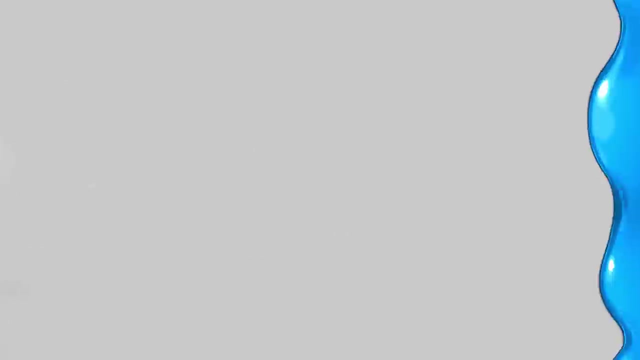 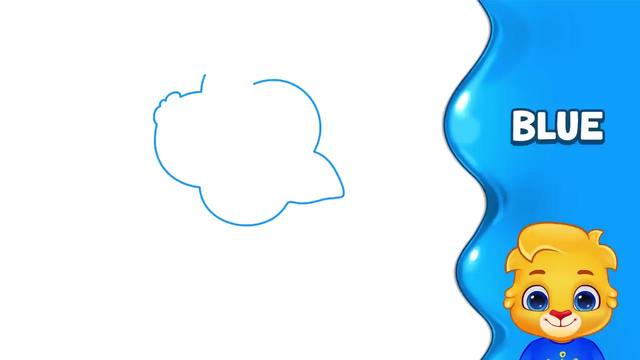 Brown Chocolate is brown Acorn. is brown Cookies. are brown Bear. is brown Box. is brown Monkey. is brown Brown chocolate. Brown acorn. Brown cookies. Brown bear- Brown box. Brown monkey. Brown box. Brown monkey. Blue Dolphin is blue. Blueberries are blue. 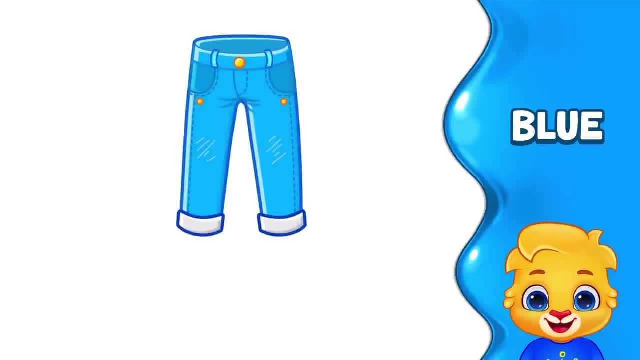 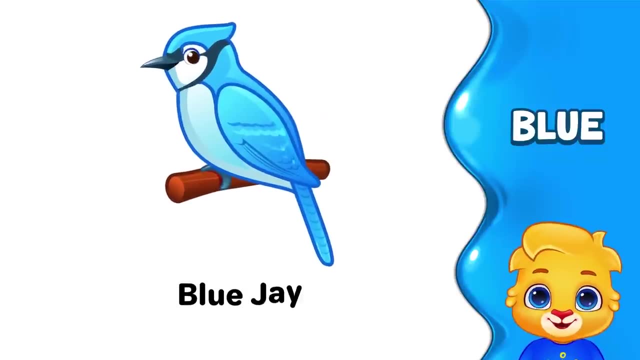 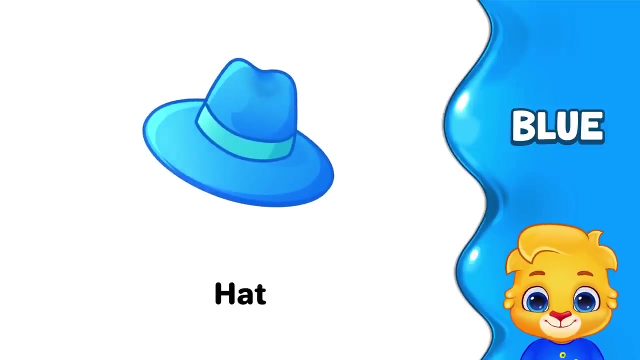 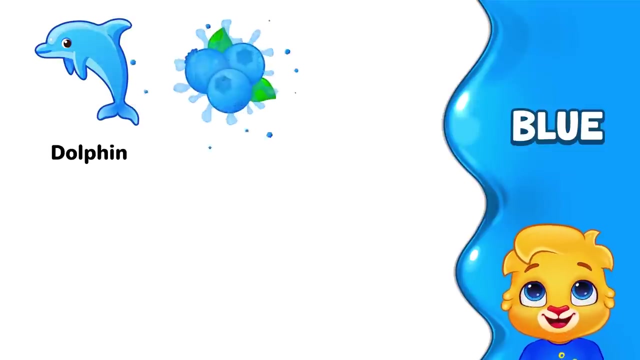 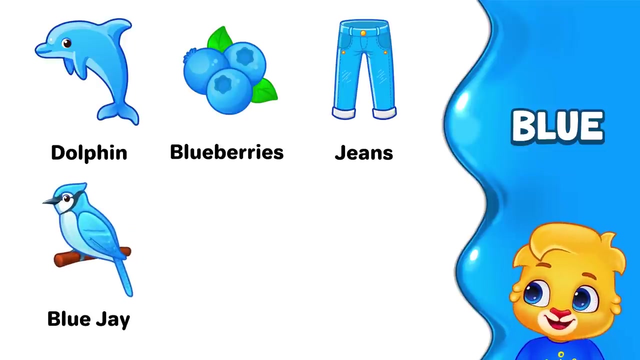 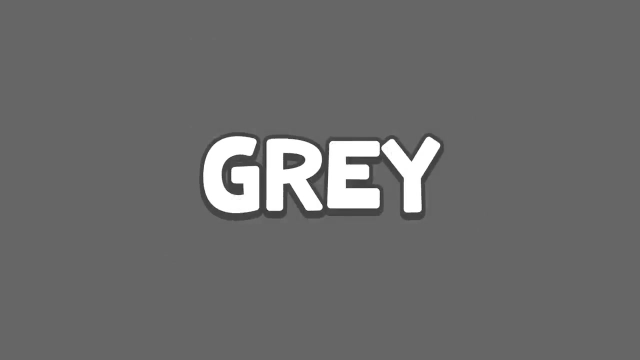 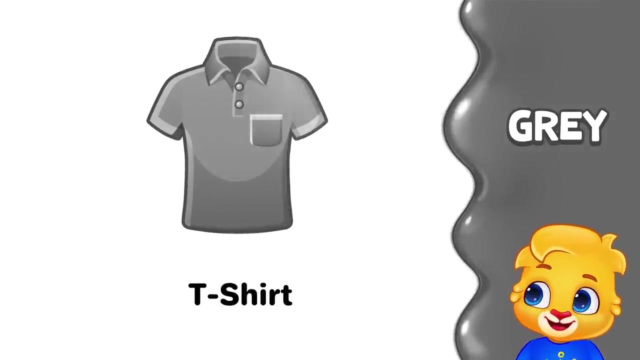 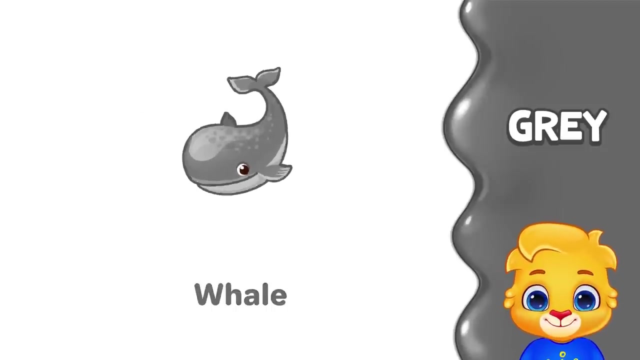 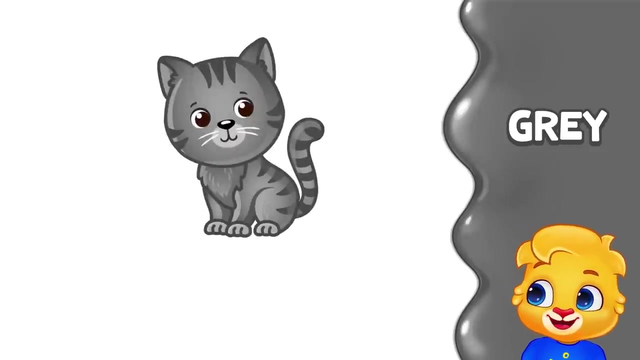 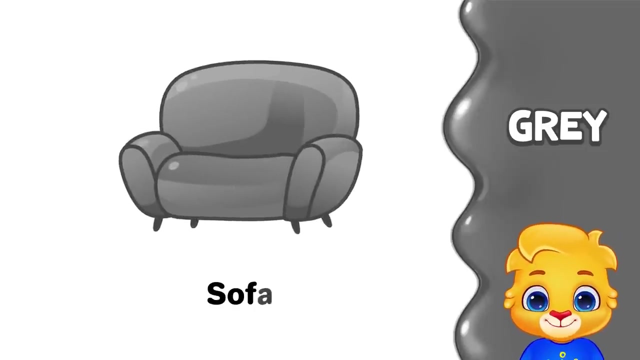 Jeans is blue. Blue jay is blue. Hat is blue. Bucket is blue. Blue. Dolphin- Blue, Blueberries- Blue Jeans, Blue, Bluejay Blue. Hat, Blue Bucket- Grey. T-shirt is grey. Whale is grey. Koala is grey. Socks is grey. Cat is grey. Sofa is grey. T-shirt is grey. 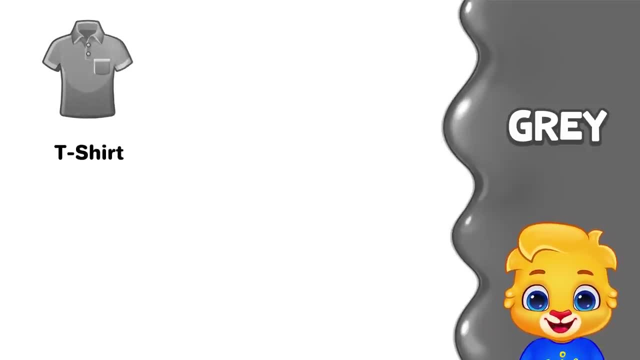 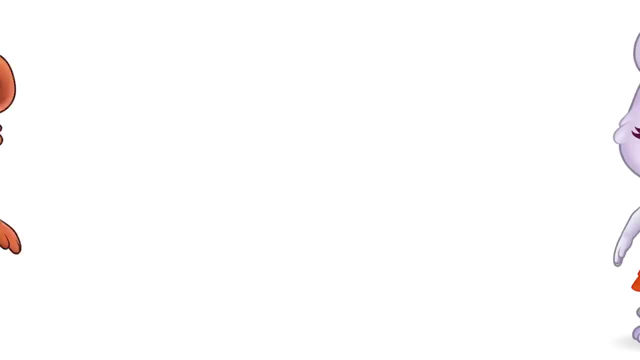 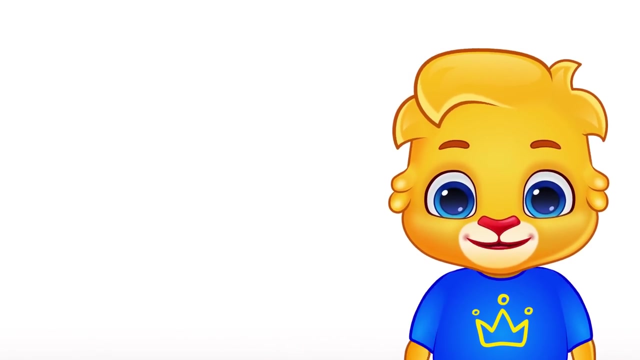 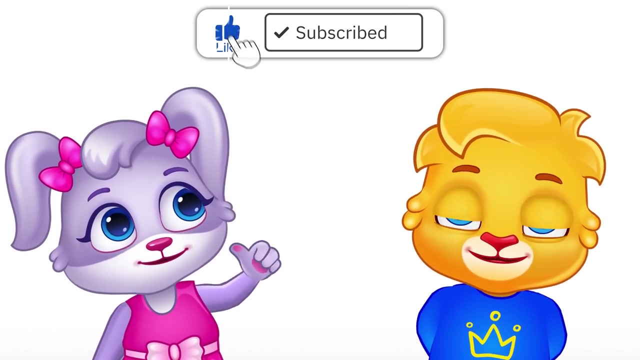 T-shirt is grey. Whale is grey. Koala is grey. Socks is grey. Cat is grey. Sofa is grey. grey Sofa is grey. fff 4: Yayyy, Suck the Hen. Hey, kiddos and parents, Hope you enjoyed the video. Can you subscribe to our channel and hit that like button? 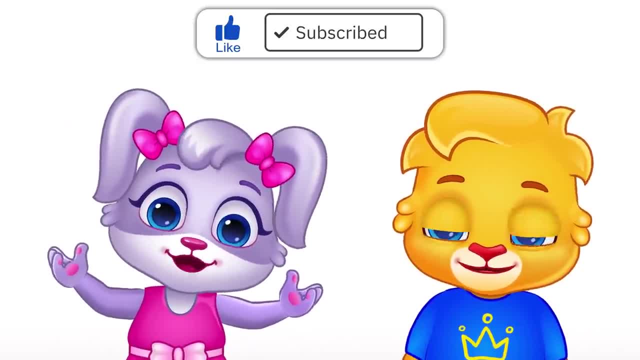 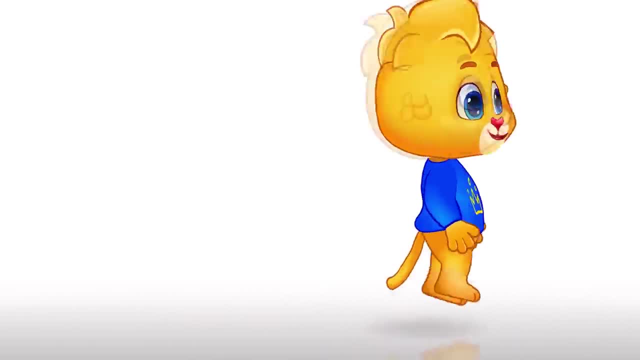 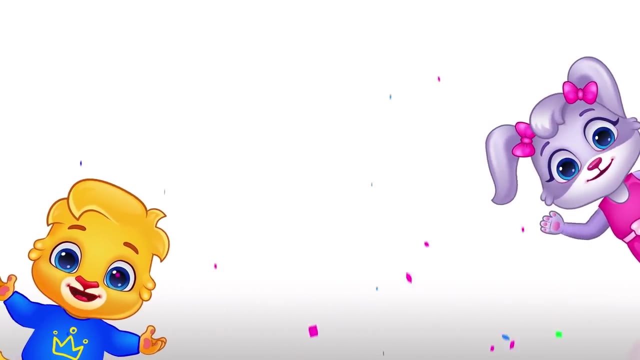 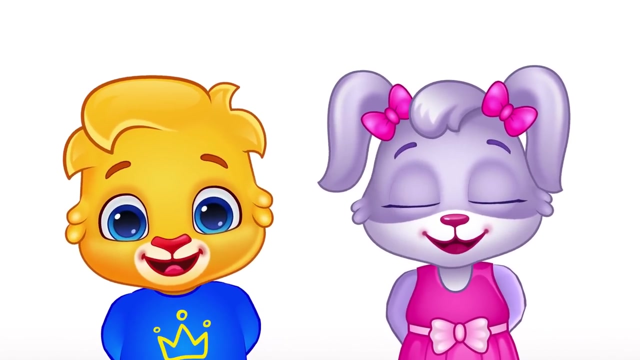 It really, really, really helps. recommend our video to other parents on YouTube. Bye-bye, Wait for me. Bye-bye, Surprise, We're back. Thanks for watching. Can you give me a big smile before I leave? Bye-bye.